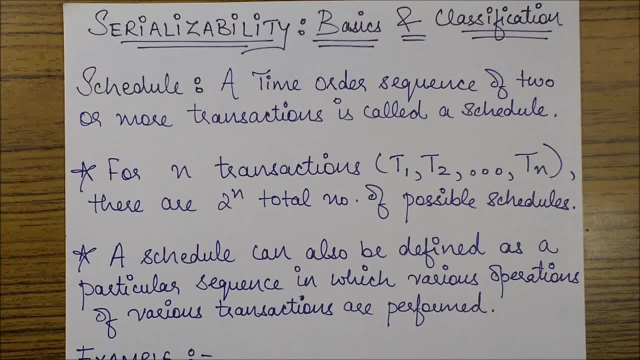 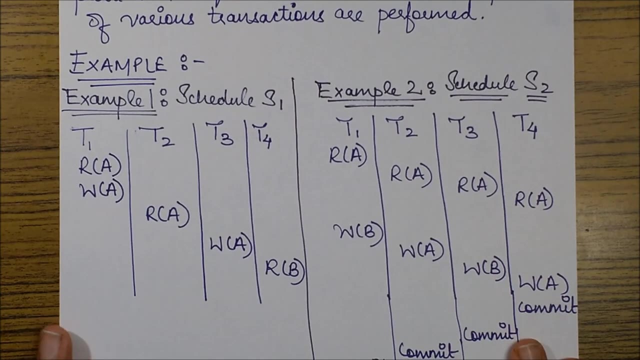 Now a schedule is termed as a time order sequence of two or more transactions. So if we have a group of transactions performing some particular function, then they are in a group or combinedly, known as a schedule. For example, we have an example of a schedule. 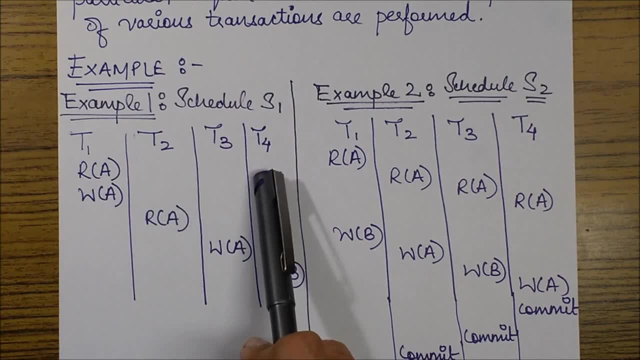 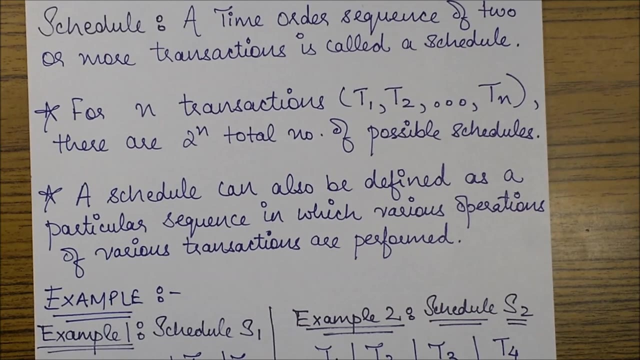 over here. This is schedule 1.. We have four transactions over here which are executing parallelly, and in this schedule 2, again we have four transactions executing parallelly. So these are the examples of schedules. Now for n transactions: t1,, t2, so on. till tn, we can say that there are 2 to the power. 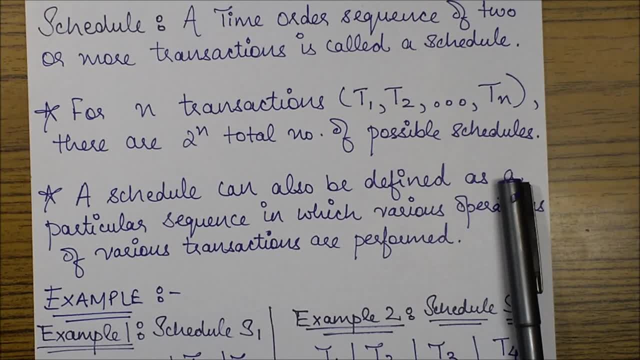 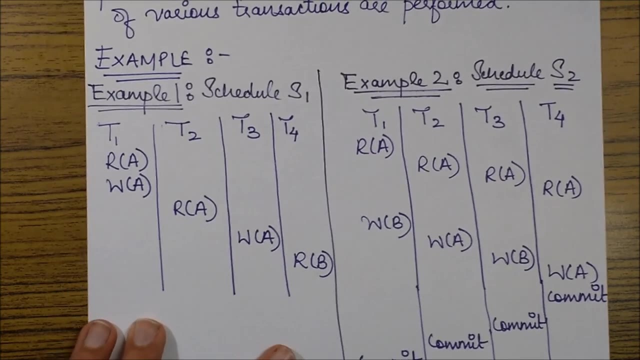 n total number of possible schedules, because there will be 2 to the power n possible combinations. Now, schedule is also defined as a particular sequence in which various operations of various transactions are performed. Let's see this clearly again: In this case the schedule does not only show that which are the parties participating. 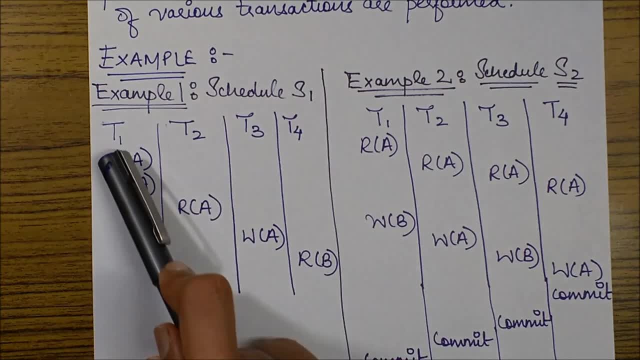 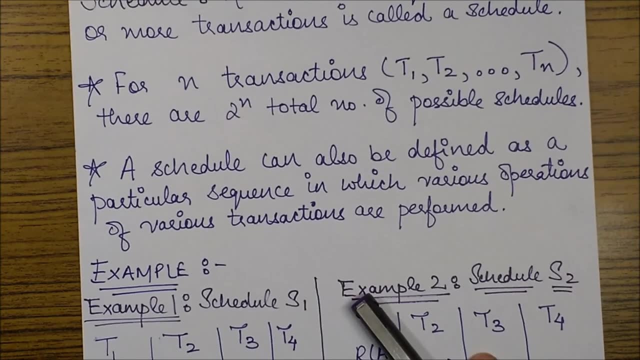 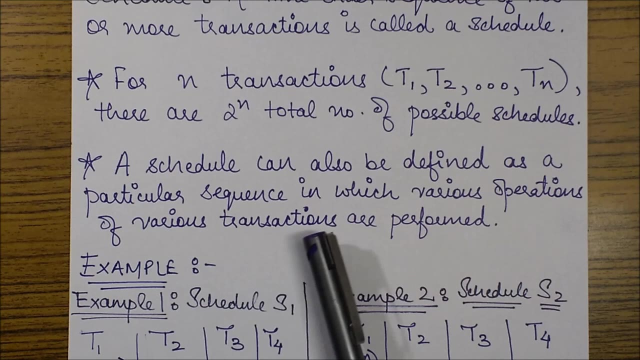 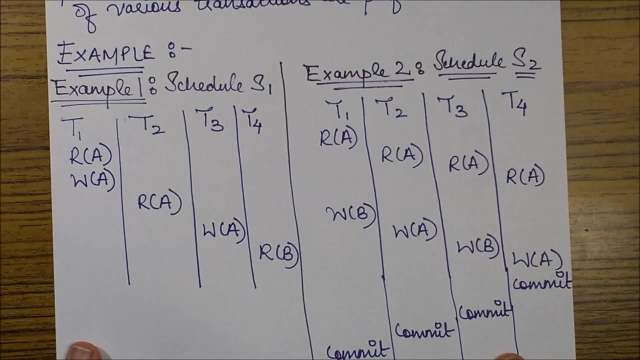 it also lists the particular sequence in which various operations for these transactions are performed. Hence we say that a schedule is defined as the particular sequence in which various operations of various transactions are performed. Now let's see the difference between the two schedules. In the first schedule we have a time order sequence. 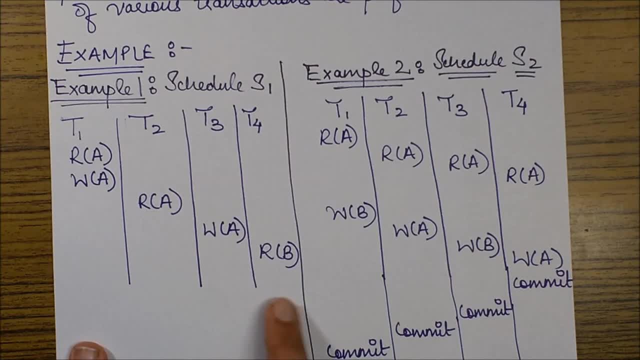 In the 2 day schedule we don't have to mention any commitment statement- GER gummet- Whereas in the second schedule we have mentioned a commit statement for all the transactions. Now we already know that what is a commit statement means. We already covered that in. 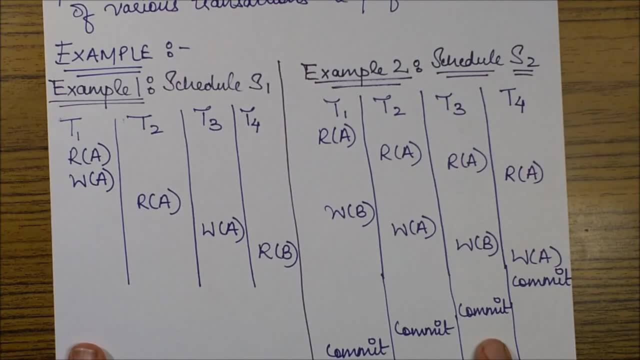 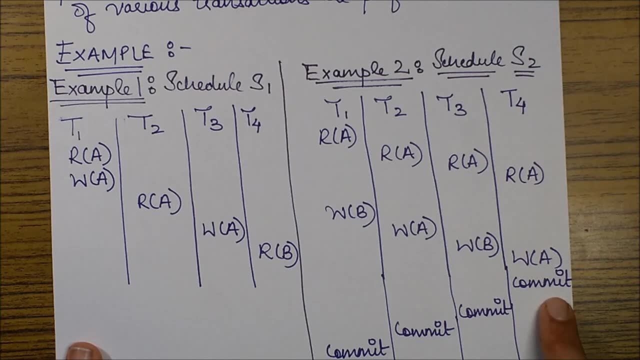 the previous session. A commit basically means that I am completing all the processes for a particular transaction, Like if I have written a commit over here. that means I am done with all the operations of this transaction. Similarly, commit of this means I am done with all operations for this transaction. 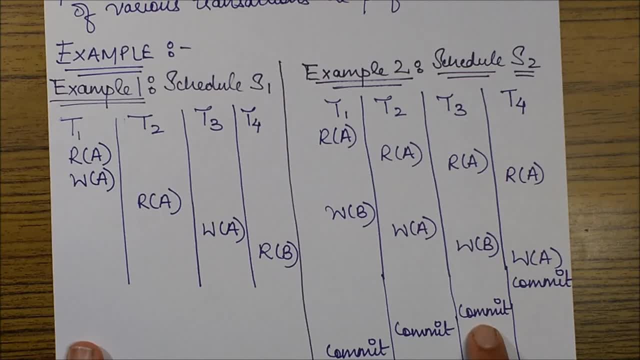 done with all the transactions, operations for this transaction. So a schedule which contains a commit or an abort operation corresponding to every transaction is known as a complete schedule. So S2 over here is a complete schedule, whereas S1 cannot be termed as a complete schedule. 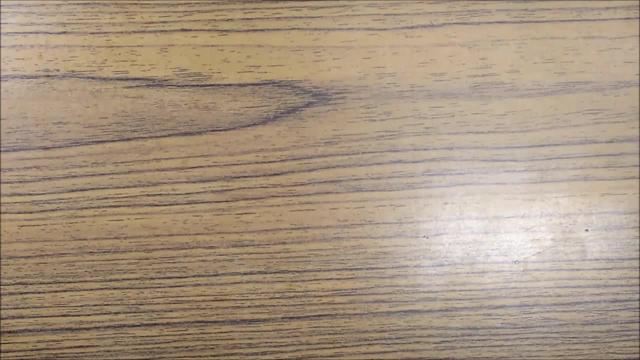 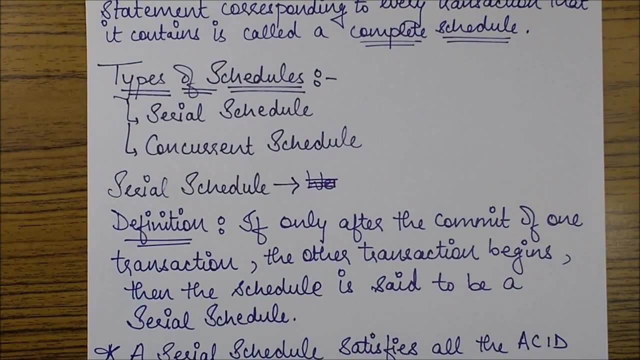 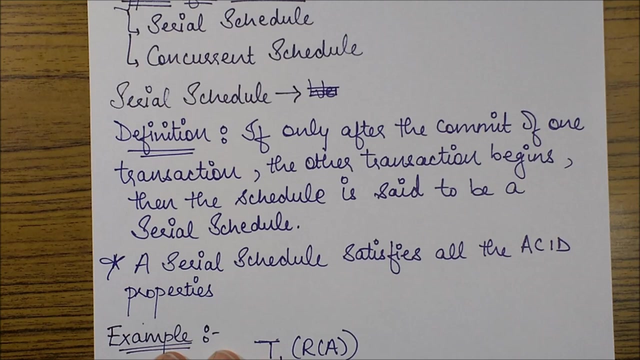 So let's move on to the types of schedules next. There are two types of schedules. We have a serial schedule and a concurrent schedule. Now let's see the definition. A serial schedule is defined as if only after the commit of one transaction the other transaction begins. then the schedule is. 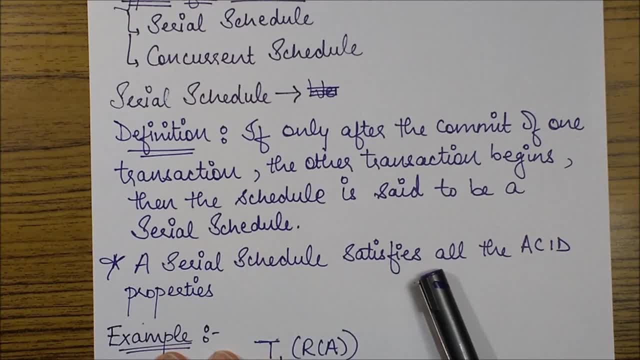 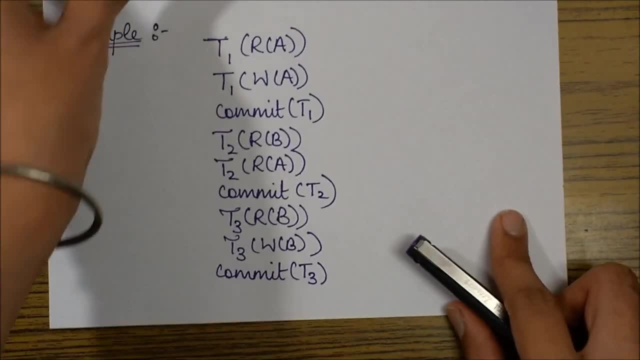 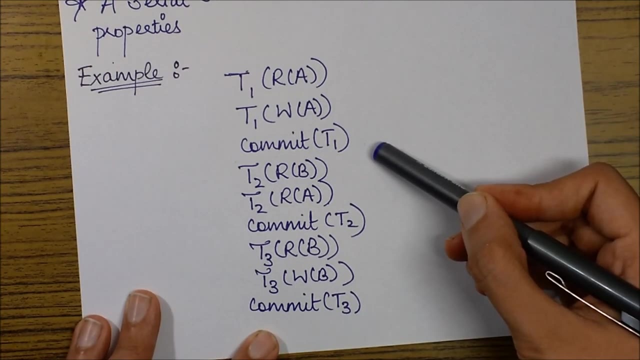 said to be a serial schedule. A serial schedule is defined as if only after the commit of one transaction the other transaction begins and satisfies all the ACID properties. Let's see an example. In this example you can see that only after I have committed the transaction T1 have I started. 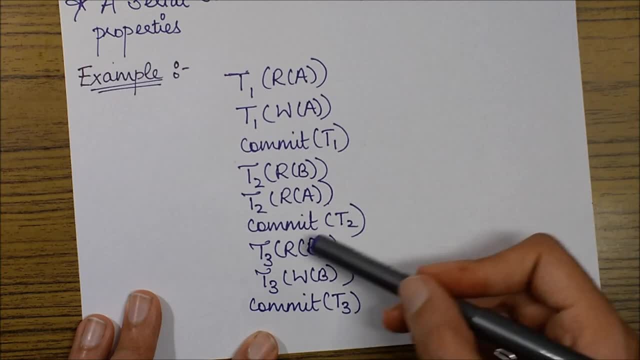 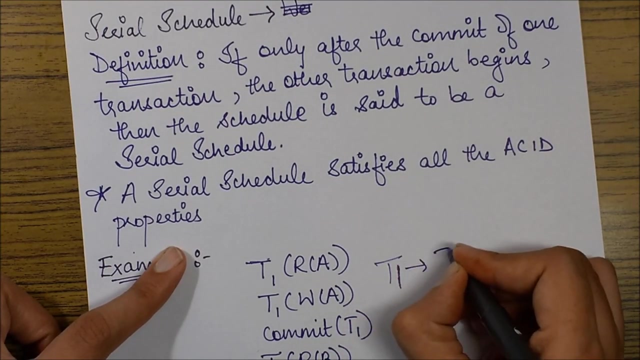 the working of T2 transaction and similarly, after the commit of T2 transaction only, I have started the working of T3 transaction. So therefore this is an example of a serial schedule, Because the order of transactions over here in this schedule would be T1, then T2 and then T3.. 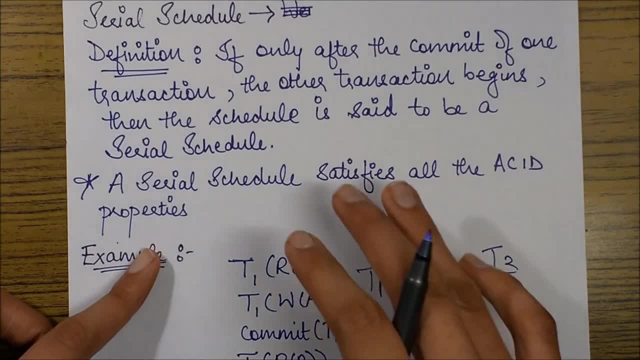 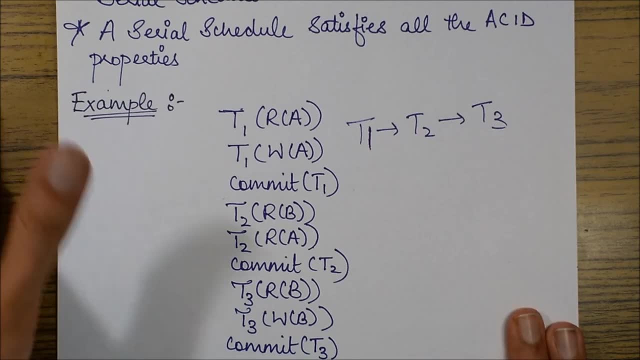 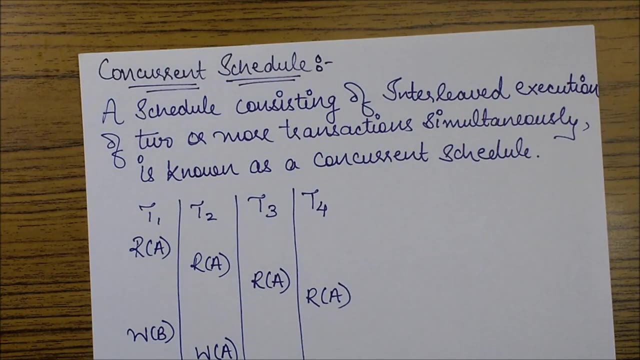 As you can see, this is a serial order. hence this schedule, this working of these transactions, is termed as a serial schedule. Now let's learn something about concurrent schedule. Now, let's learn something about concurrent schedule. already saw an example in the previous session, but let's clearly define it now. a schedule which 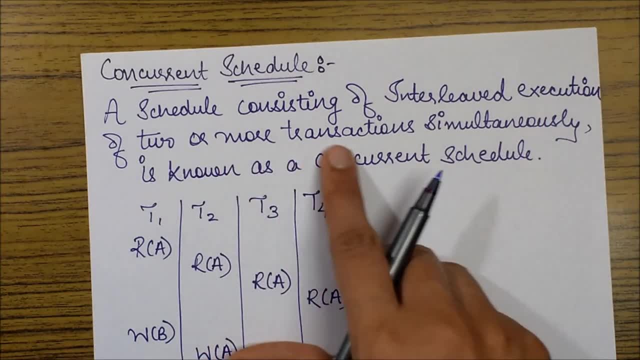 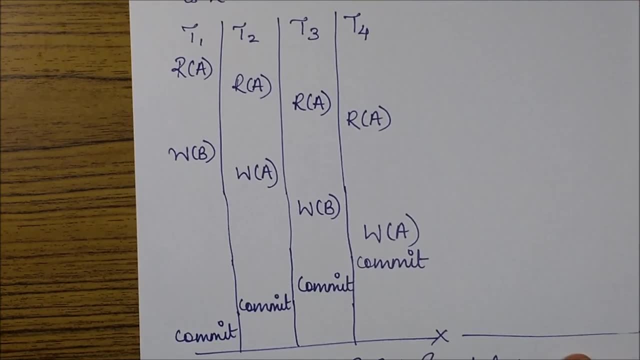 consists of interleaved execution of two or more transactions simultaneously is known as a concurrent schedule. let's see an example. in this case we have four transactions- t1, t2, t3, t4- which have certain operations over here, and we can see that they are operating parallelly. how 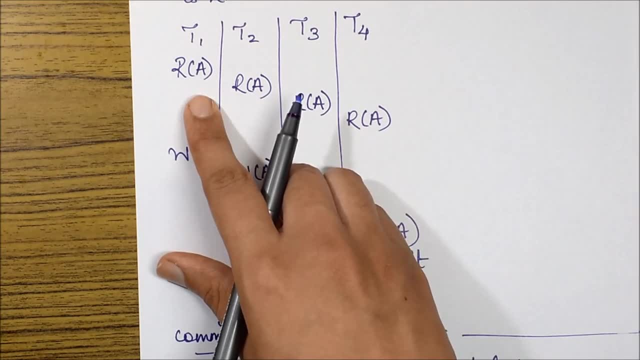 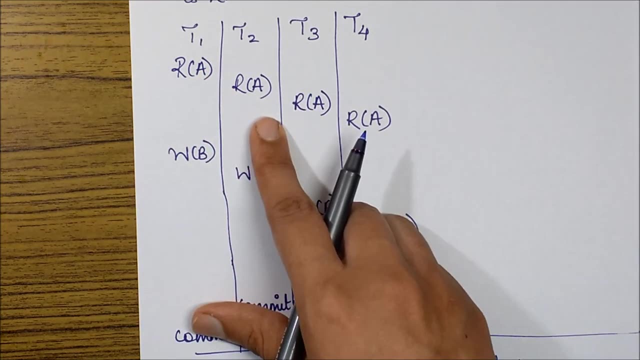 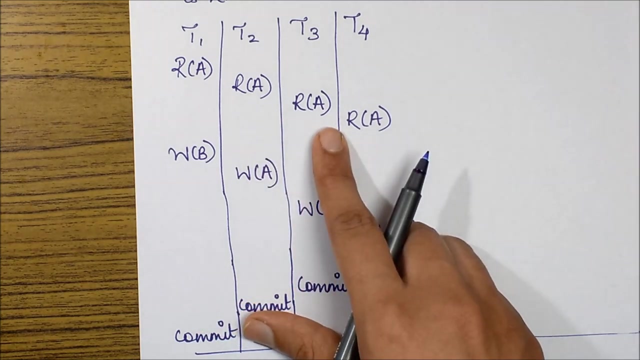 can we say that? see, first of all we operate this r1 operation, r operation, read operation on item a for t1 transaction. then we transfer the control to t2 transaction, which performs the read operation on this item a, then the control is transferred to t3, then to t4 and then again the control is. 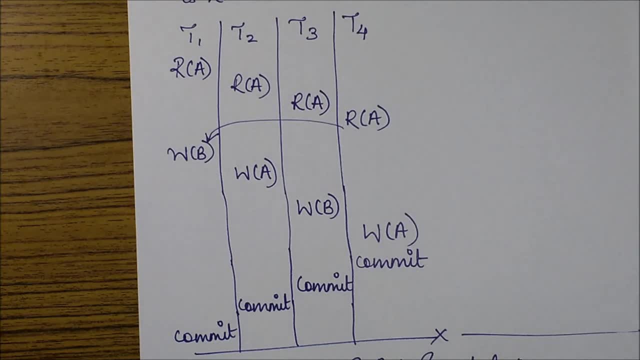 transferred to t1. so as the control transfer is being done within this particular schedule, we say it is a concurrent execution or a parallel execution. hence, this is an example of a concurrent schedule. also, since a commit has been listed for each and every transaction, this is also an example. 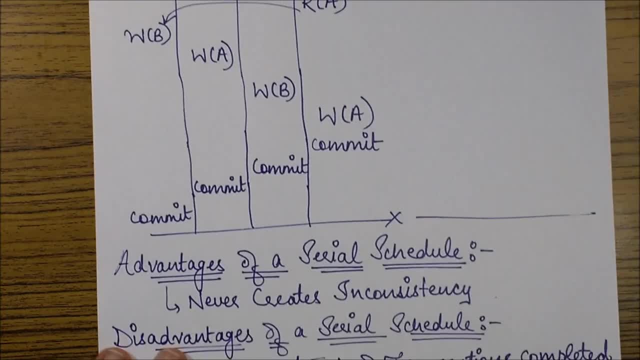 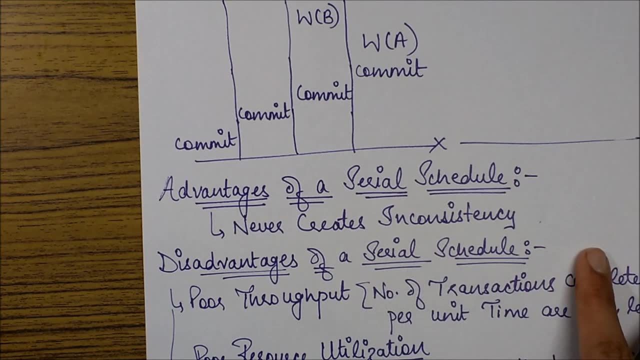 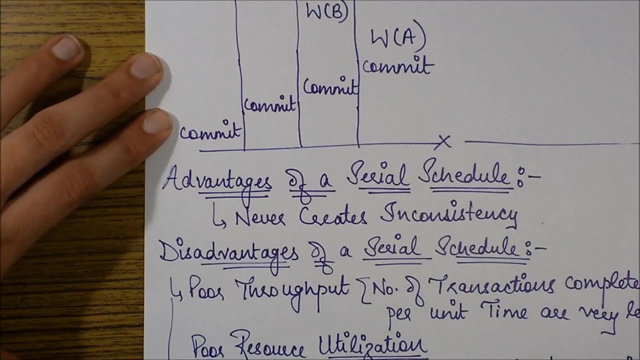 of a complete schedule. now let's see the advantages and disadvantages in both the cases. the advantages of a serial schedule are: it never creates inconsistency because it satisfies all the ACID properties. now the disadvantages are as follows: we get a poor throughput because number of transactions completed per unit time are very 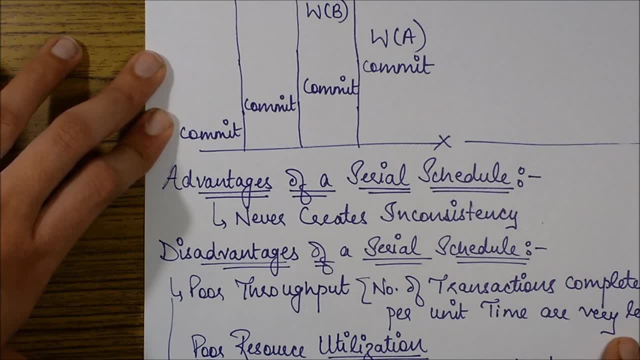 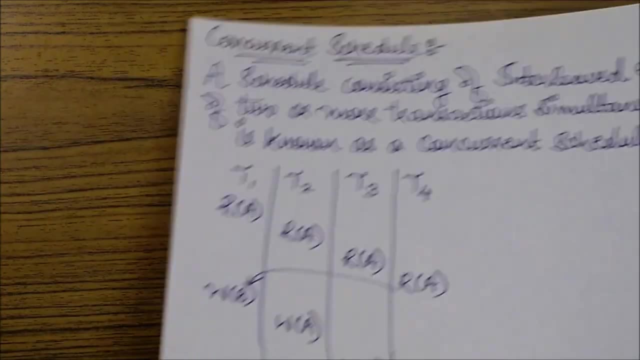 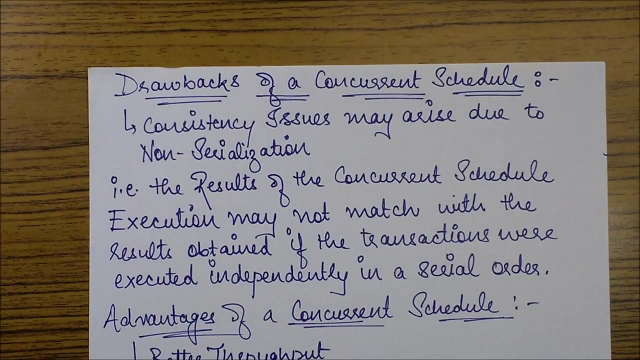 less. this is because at any particular instant of time only one particular transaction is executing. then there is a poor utilization of resources. this is because there is no sharing of resources among various transactions. now let's see the drawbacks in case of a concurrent schedule. the consistency issues are there because, since there is a parallel execution of the transactions, we cannot 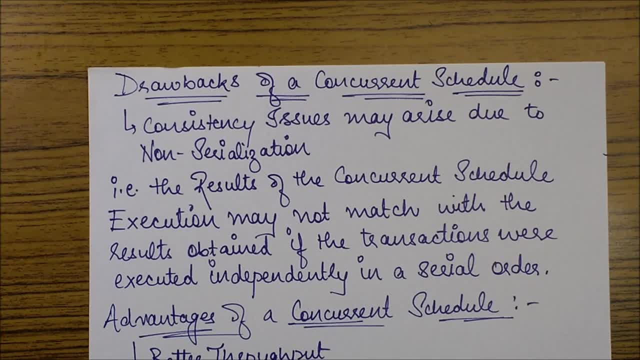 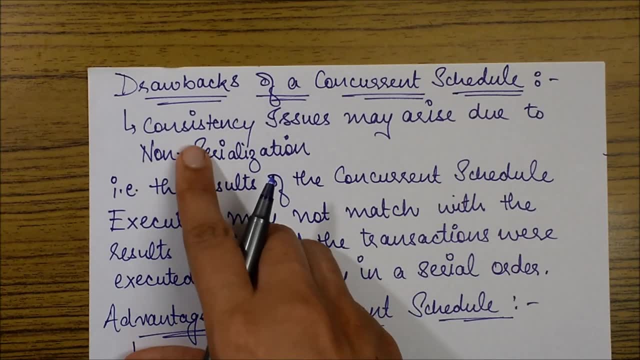 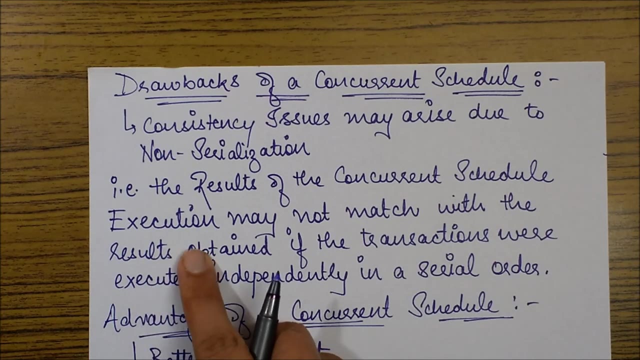 say that all the ACID properties will necessarily be satisfied. so we have to ensure that all the ACID properties are satisfied. so that means there is a chance of inconsistency in this case, that is, the results of the concurrent schedule execution may not match with the results obtained if the 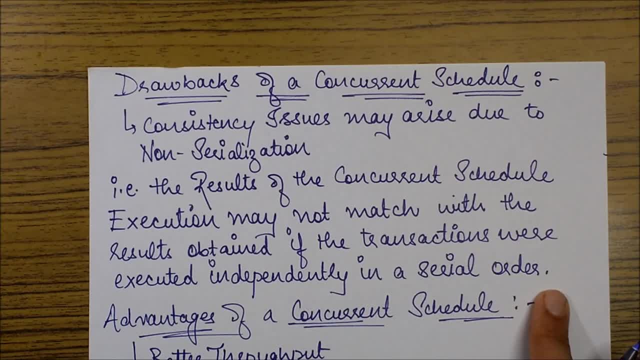 transactions were executed in the current schedule. so that means there is a chance of inconsistency in the current schedule. so that means there is a chance of inconsistency in the current schedule. so that means there is a chance of inconsistency in the serial order. but there are also certain advantages. what are those advantages? we certainly get a better 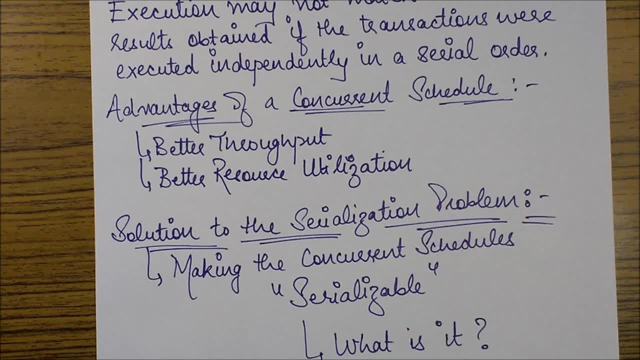 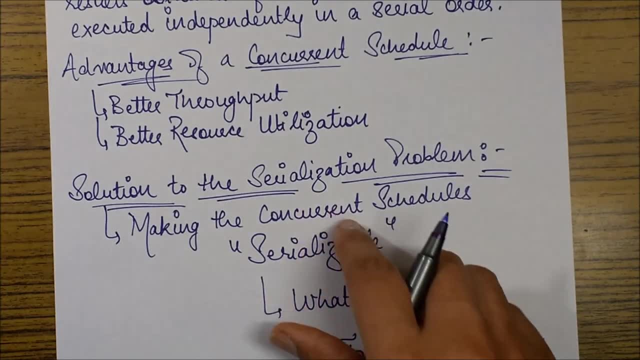 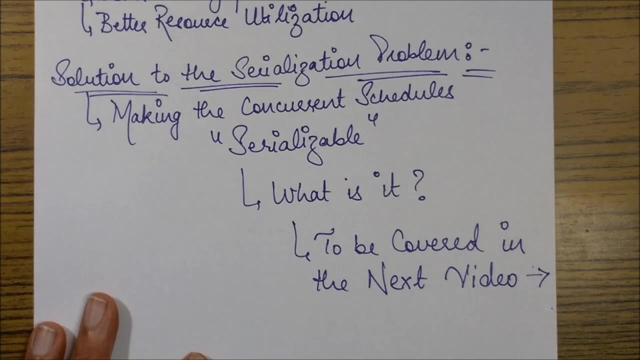 throughput and a better resource utilization. now, what is the solution to this serialization problem? then, the solution is serializability. so what is the solution to this incurrency problem? it is serializability. and how do we do it? do it, we'll see that in the next video, so see you all in the